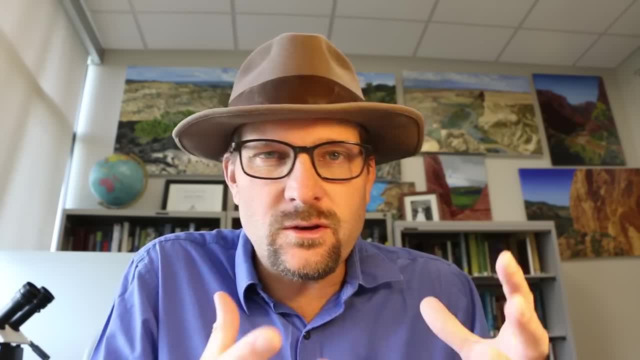 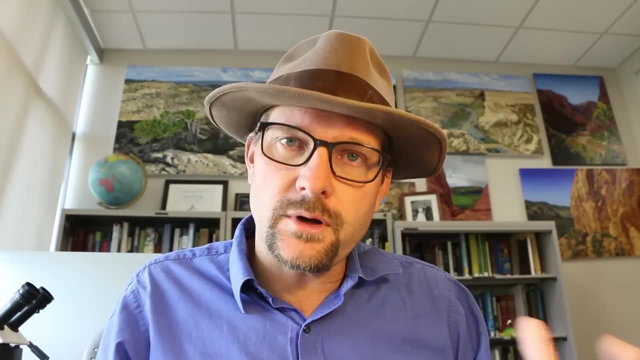 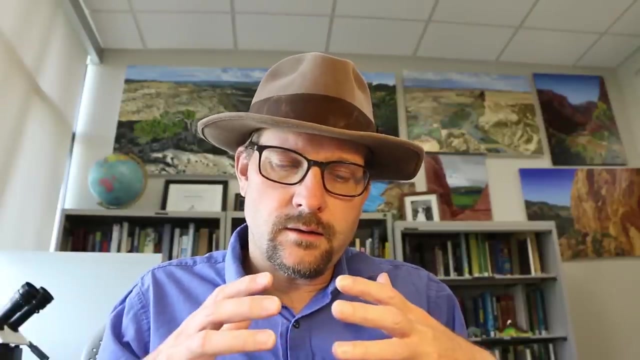 animals and plants. I want to work either in the field collecting fossils or at a natural history museum, and I just love dinosaurs and other prehistoric animals. how do I make a career doing that? In this video and the next video, I will help guide you on the steps and discuss what to 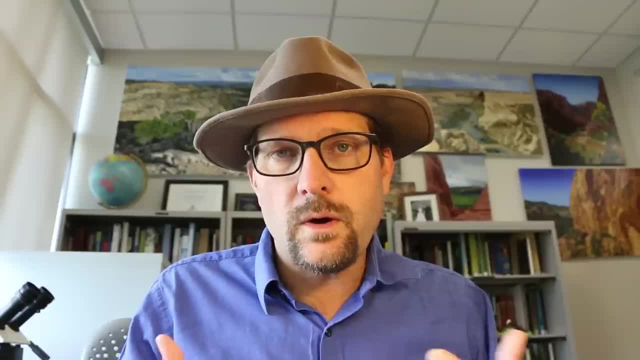 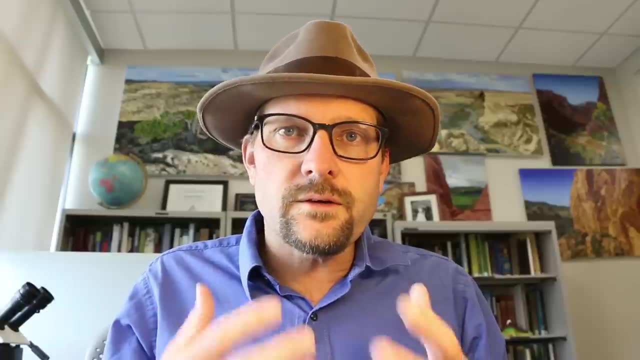 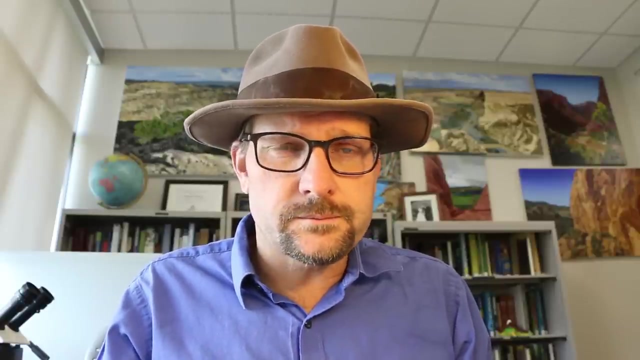 study the various classes you should take and what education you might need as a paleontologist. In a second video I will post next week I will discuss the different types of jobs in paleontology. So if you are still in high school, middle school, junior high or elementary school, 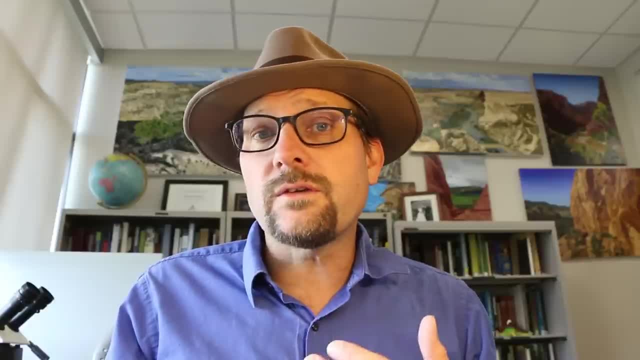 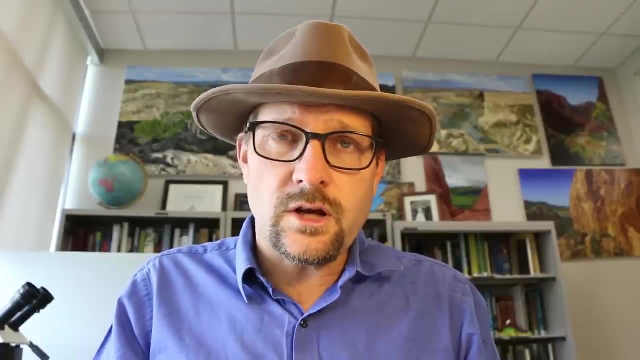 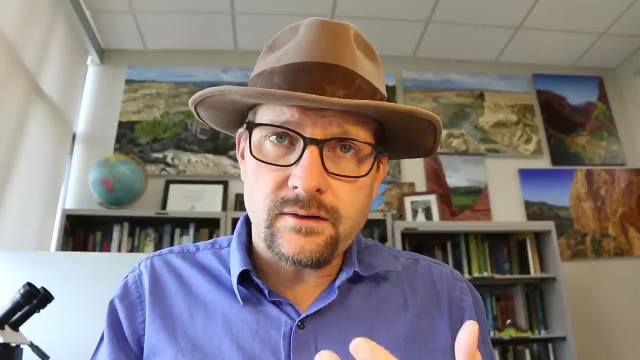 you want to do well in all of your classes and if, given the choice, you want to take as many science classes that you can Now, I recommend that you should take at least a year of geology, biology, chemistry and physics. Some states here in the United States lack some of these sciences at the high school. 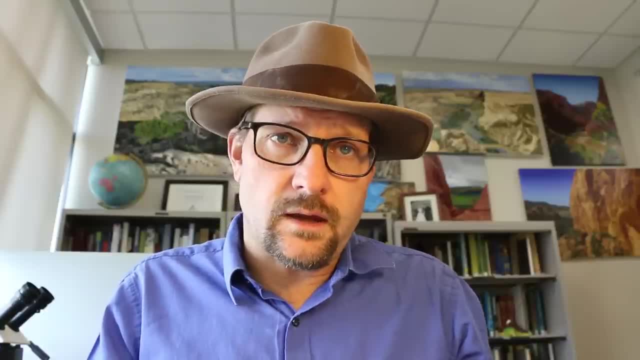 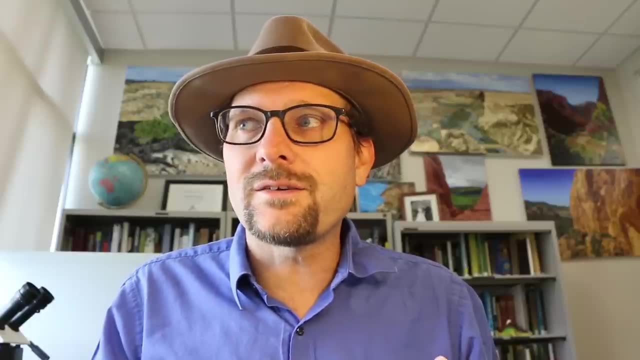 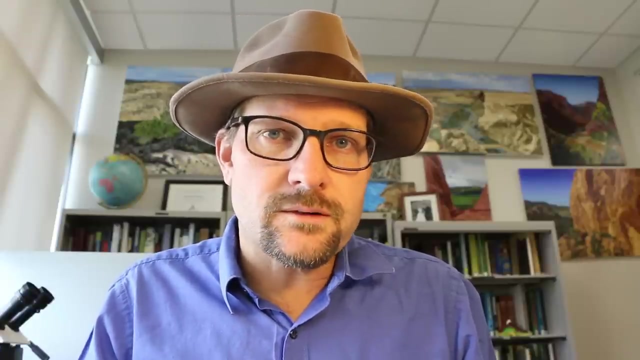 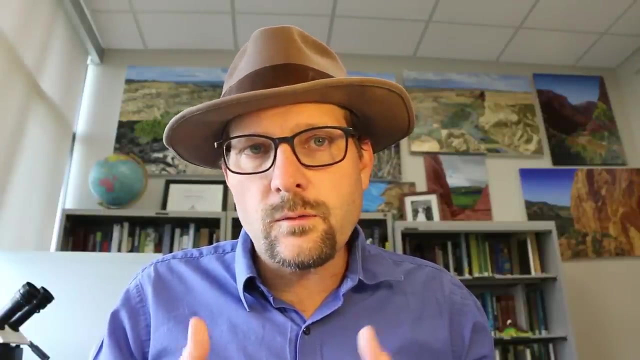 level. You should supplement this with books if you can, so you should read as many science books on paleontology and spend time learning about rocks and minerals and animals and plants that you are most interested in studying by reading books. Now, to be a paleontologist, you really need to attend a college or university and selecting 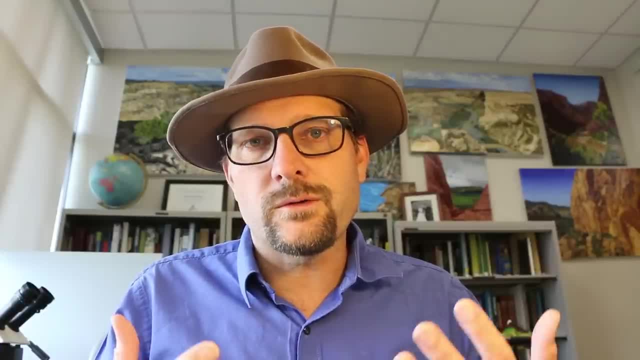 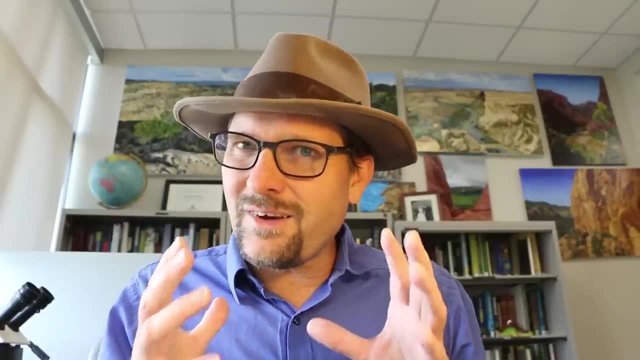 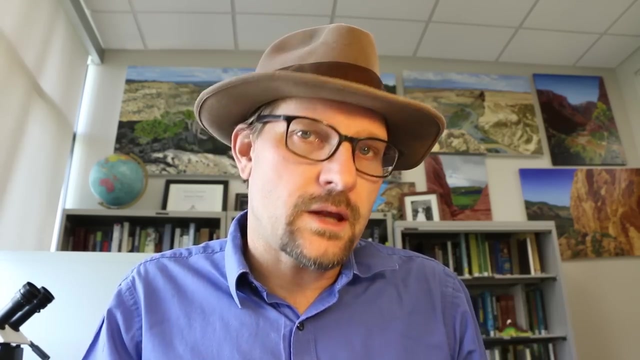 the right place to continue your studies is one of the most critical decisions that you will make Now. if you are switching careers, it may be a little daunting considering returning back to college, but it is basically the best way to get into a paid paleontology job. 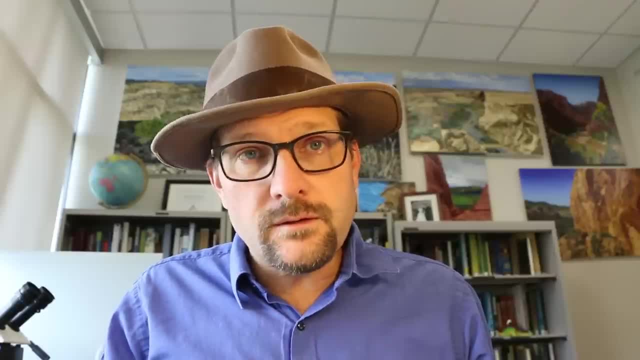 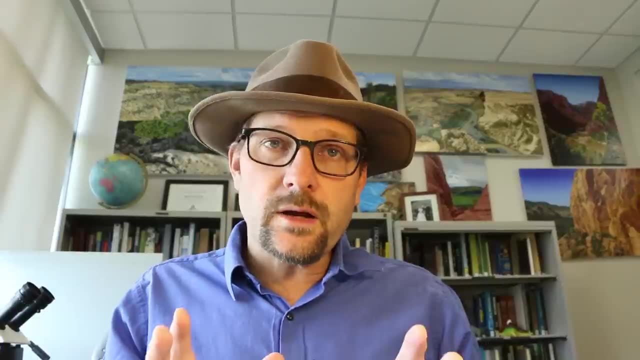 But if you don't have the time or resources, volunteering at a natural history museum may be the best avenue to get you into the paleontology field. Now, I highly recommend not attending a community college, vocational or technical school, since these schools lack instructors. 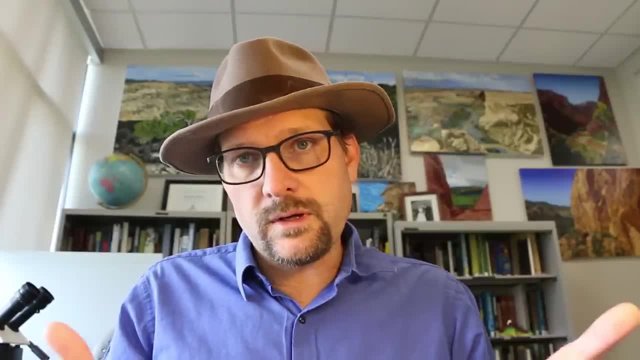 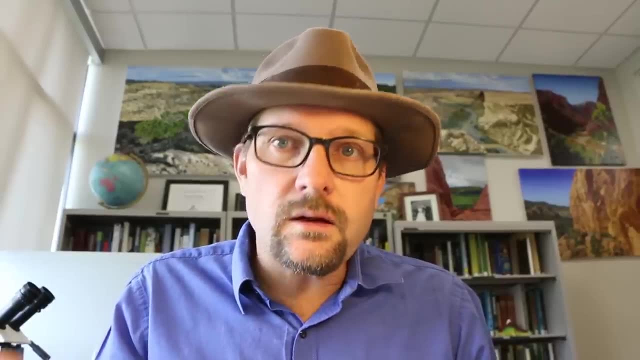 I have a few examples of some of the top instructors that you would need for a well-rounded program. for an aspiring paleontologist, It might be tempting, since these classes at these schools are often cheaper, but it is not going to be very useful for you. 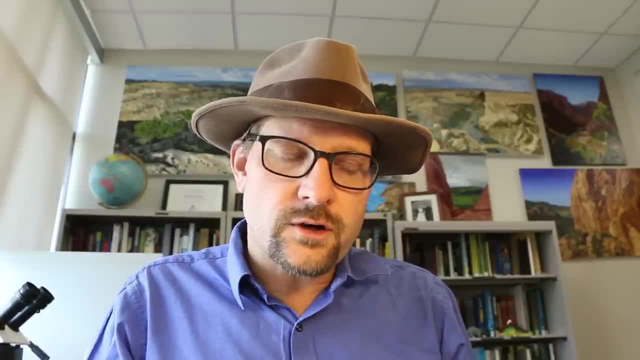 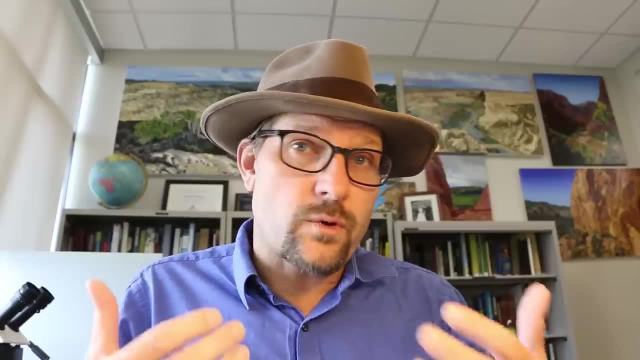 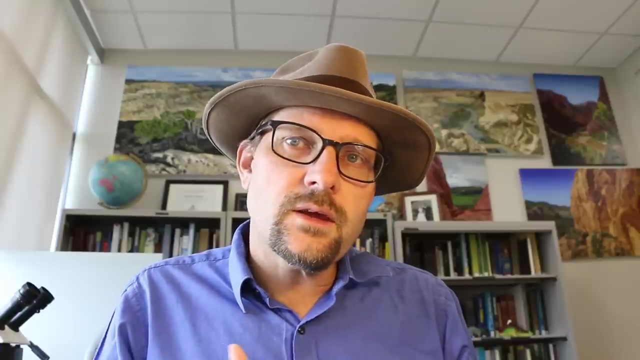 So look for colleges that have at least one instructor or professor who teaches paleontology. Ask the university or college if those classes are taught regularly and try to find out about the instructors and how well-respected they are in the field. Another key thing is to look to see if they have an associated natural history museum. 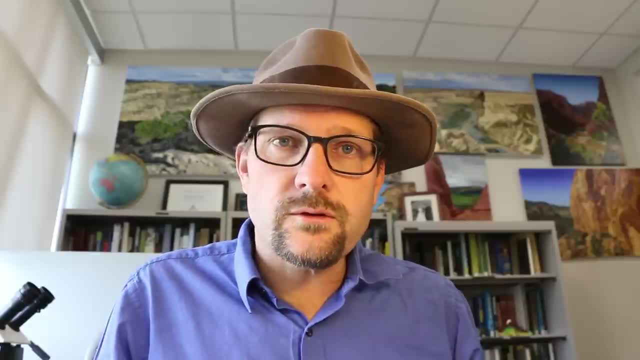 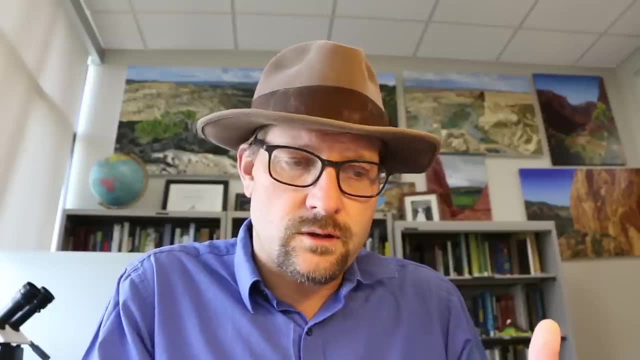 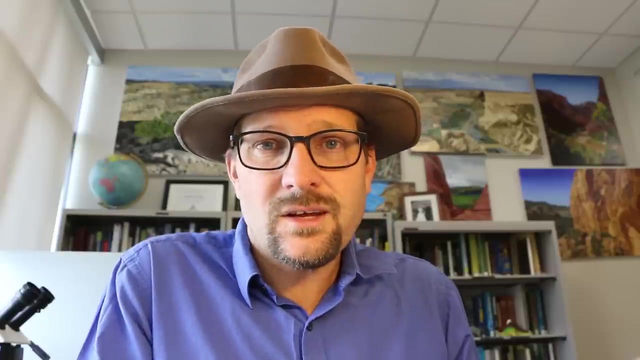 within the university Here at Utah State we have the Prehistoric Museum in Price, Utah. So a university museum gives some experiences to you that you can volunteer at the museum. you can learn fossil preparation, you can learn fossil collection and you can hang. 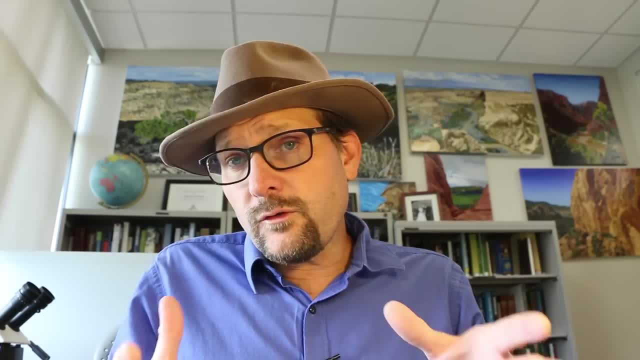 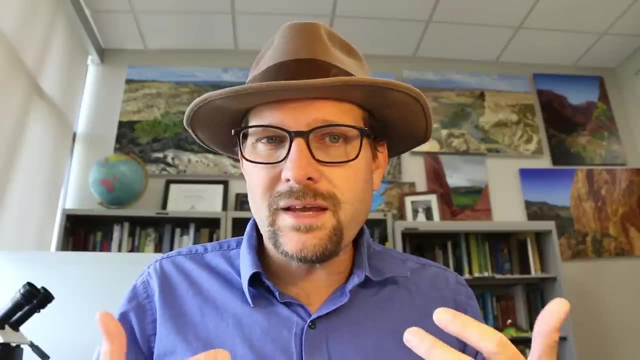 out with other aspiring paleontologists. Now, after you have applied and been accepted, and you have selected the college that you are going to enroll in, you will need to make the next big decision, and that is what major you would like to pursue. 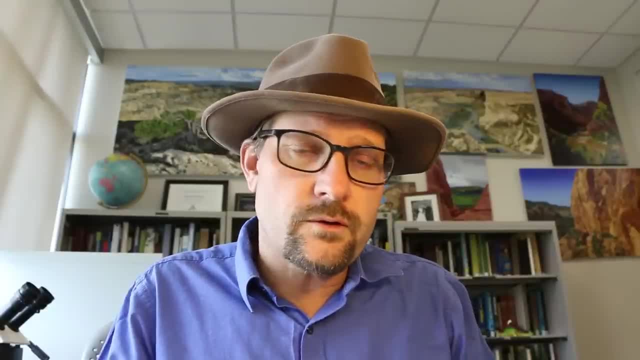 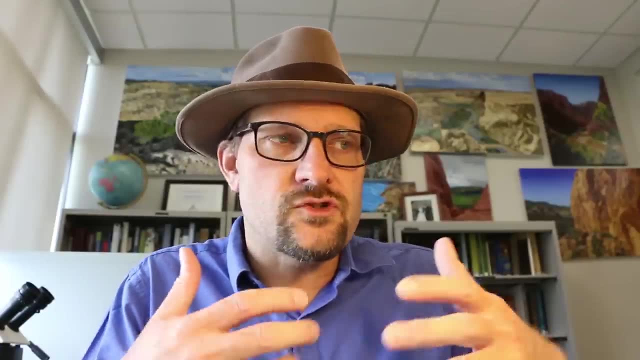 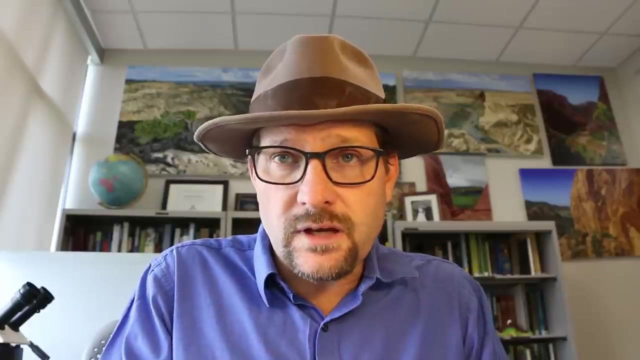 Paleontology is not offered as a major at any college or university here in the United States that I am aware of. Rather, it is often wrapped up in either the geology department or biology department, And it really depends on the university And the specialization of individual professors in each department. 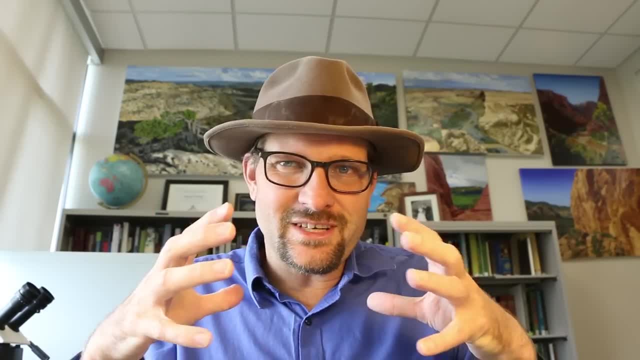 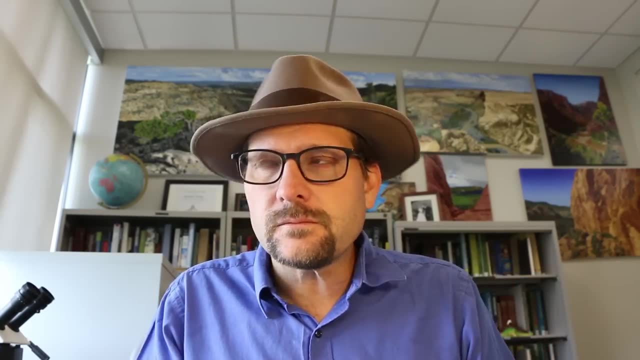 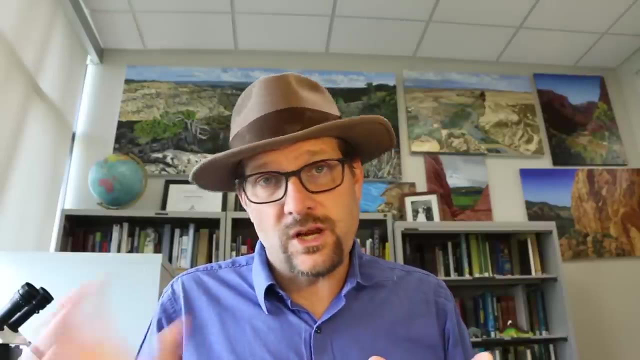 Now more and more universities are kind of pushing paleontology into the biological sciences, As those departments tend to attract more students. however, here at Utah State University, paleontology is within the geology department. Now, as a biology or geology student, you will take classes in both disciplines. 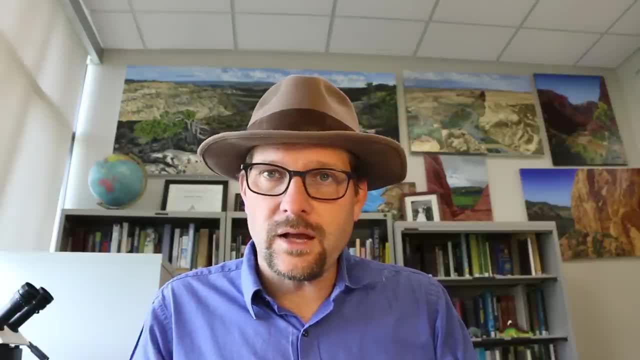 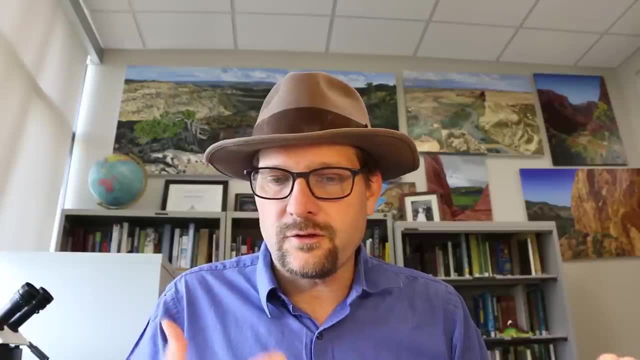 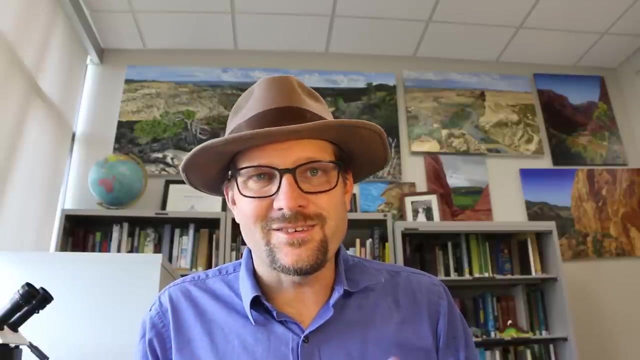 And so you want to program a study that is flexible, To take those classes that would be most useful to you. It also depends kind of on your own passion whether you want to be a biology or geology major. So if you are more on the rock side of paleontology, go on to the geology side. 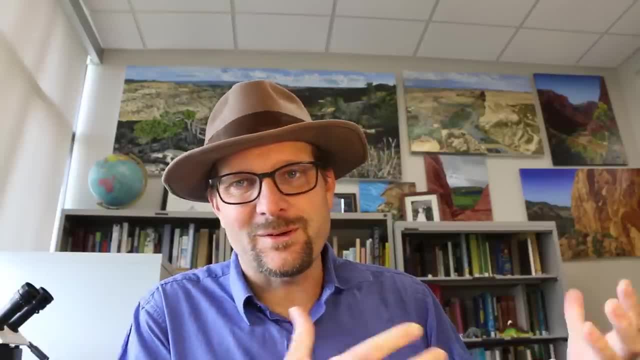 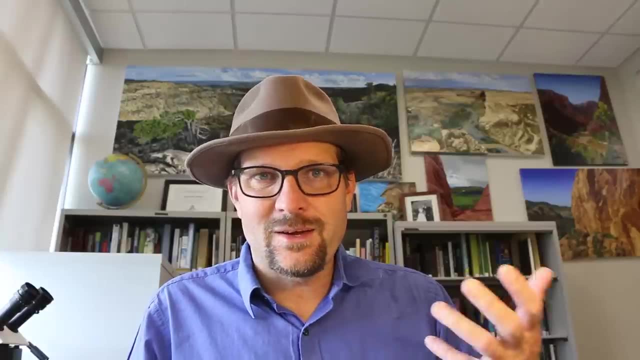 If you are more on the fleshy tissue side of paleontology, go into biology. So if you love cracking rocks open and looking inside, or do you like cracking dead animals open and looking inside? This kind of depends on your own passion. 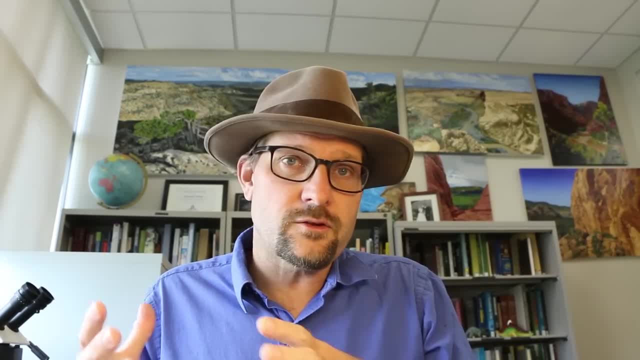 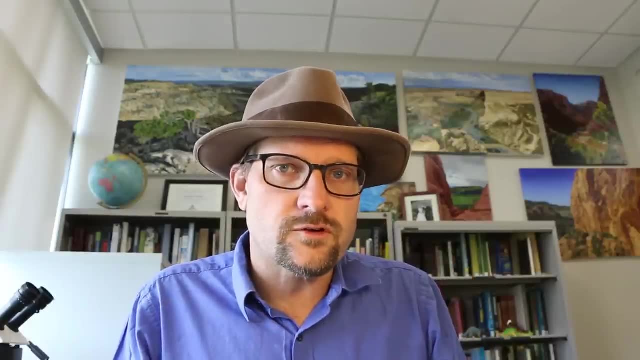 Now. this decision- whether you want to be a geology or biology major- may affect your job prospects when you graduate, So you want to think about this. It's an important decision Now. the most important classes start actually in the first year of college, with the three 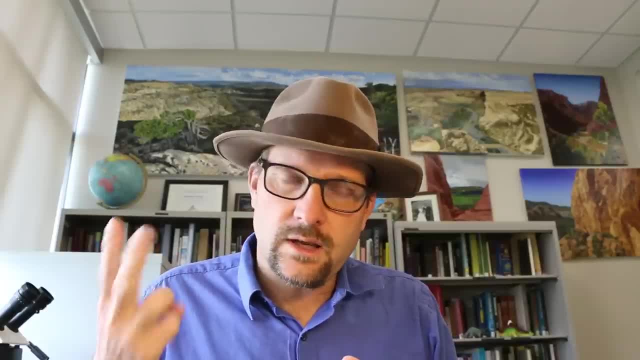 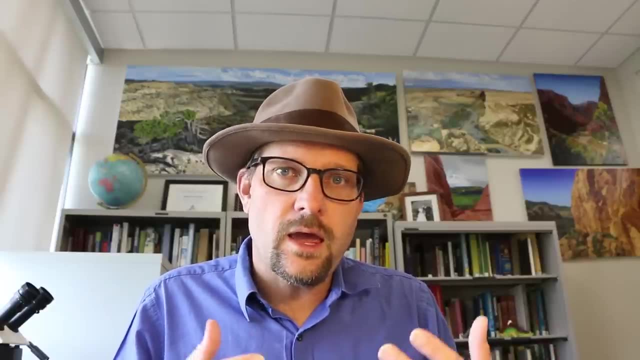 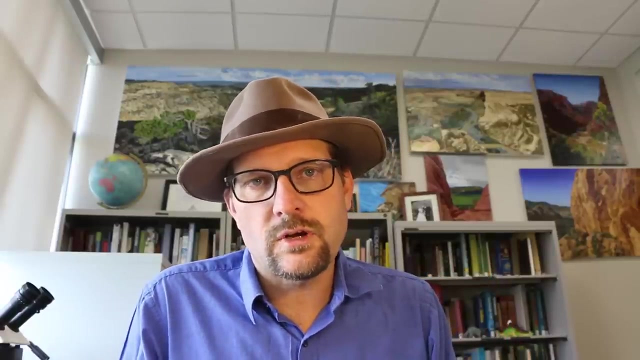 basic sciences: geology, biology and chemistry. Those will often come with really lengthy labs that will require a lot of studying work to master, But they are really a great basis for the upper division classes that you will take later in college. Also, get through any of the math requirements very early in college. 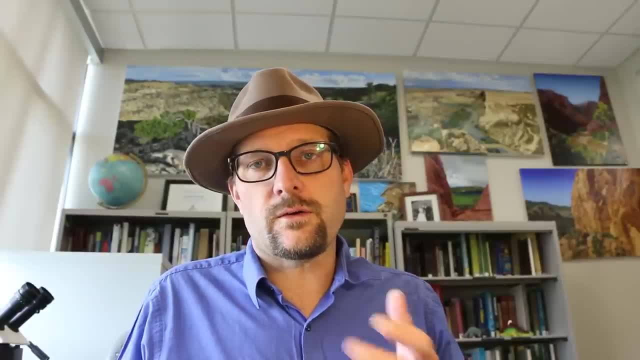 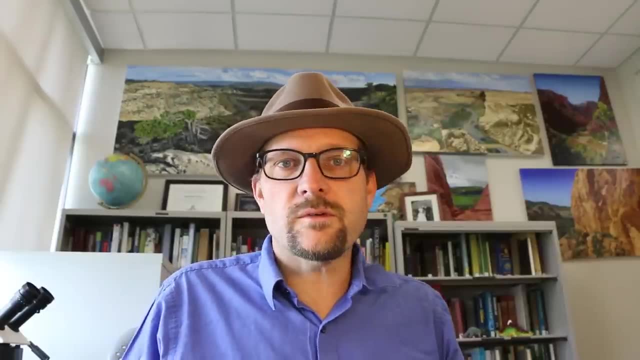 Paleontology as a class is often taken in the second year or third year of your program. It's often taught in geology departments with a focus on invertebrate fossils, sometimes paired with vertebrate paleontology. When you take the paleontology class, 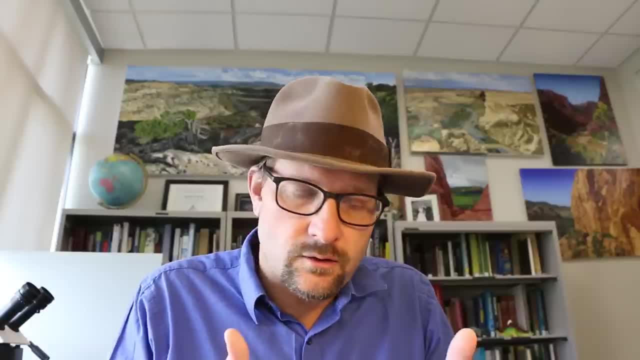 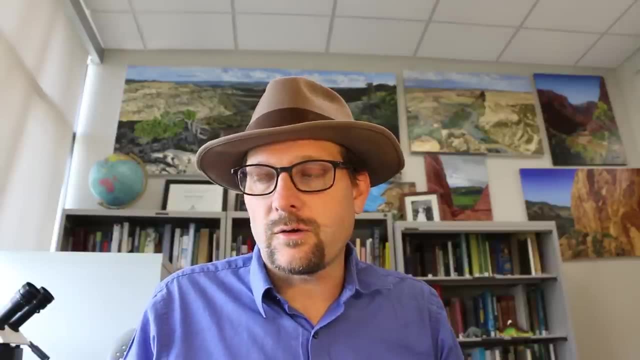 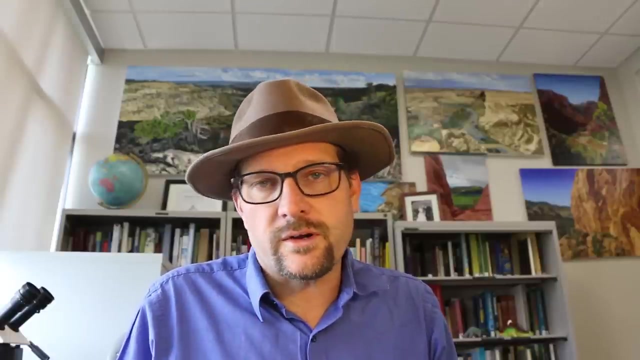 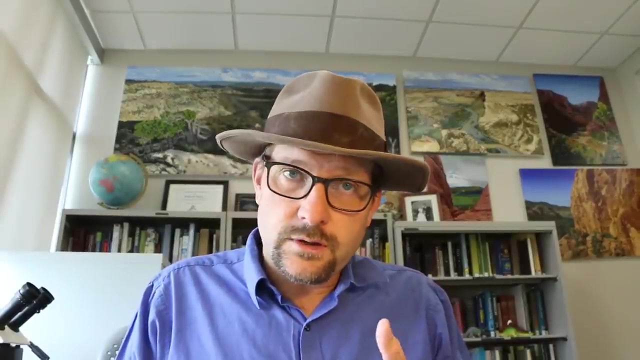 Contact the professor and meet with them to discuss your interests in paleontology, And they will likely know of resources such as field work at an active dig site, graduate students needing volunteers or undergraduate research opportunities that you can get more experience with. Other more advanced geology classes that you should take and master are Geochemistry, Mineralogy. 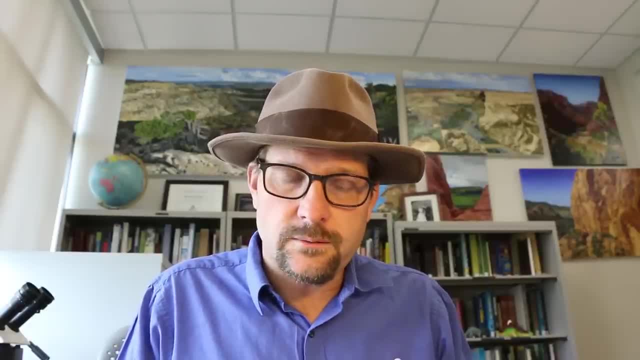 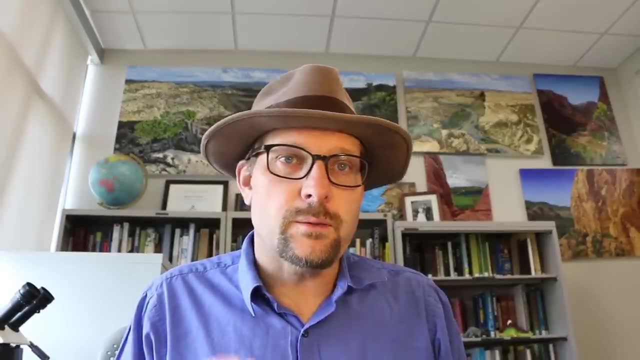 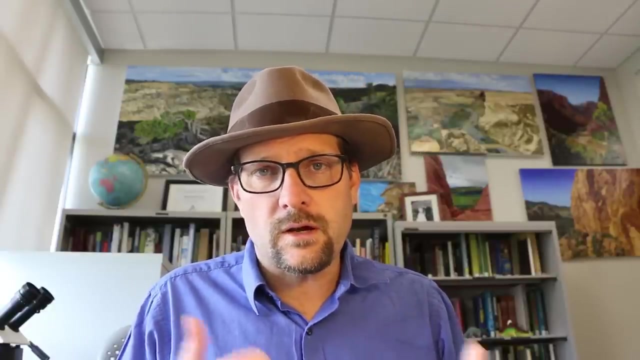 and Petrology, Sedimentary geology And Stratigraphy. You should also think about other useful classes that might be offered, like paleoclimatology, oceanography and geomorphology. Those might be useful to you, depending on your interests In biology, advanced classes you should take and master. it kind of depends on the fossil. 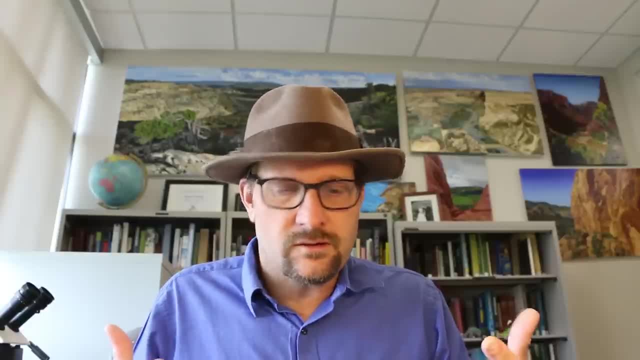 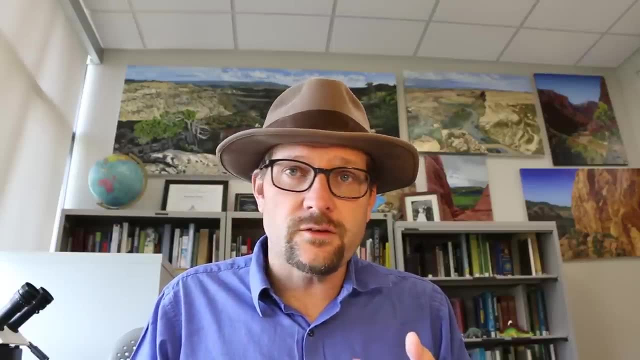 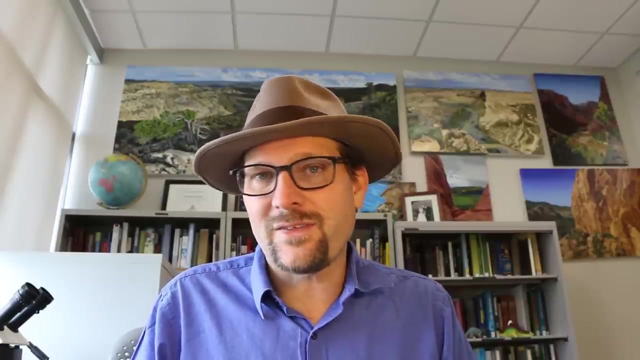 organisms that you find most interesting. But if you are interested in, like, say, dinosaurs or other prehistoric animals, courses in anatomy- imperative vertebrate anatomy, osteology, embryology, evolution, ecology, herpetology, ornithology, mammology and ichthyology would be very useful. 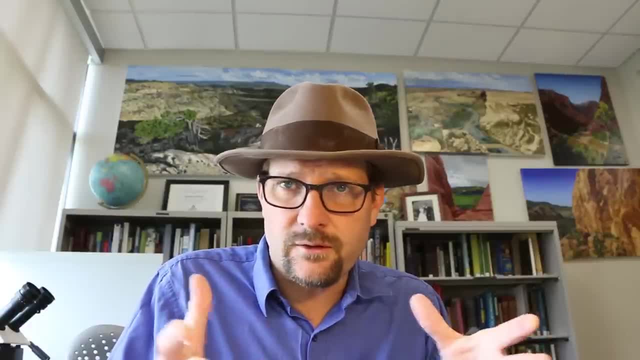 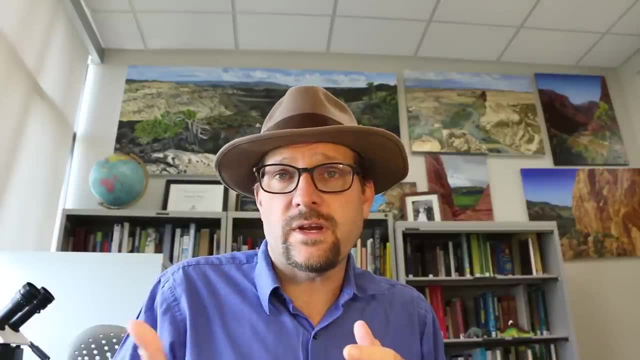 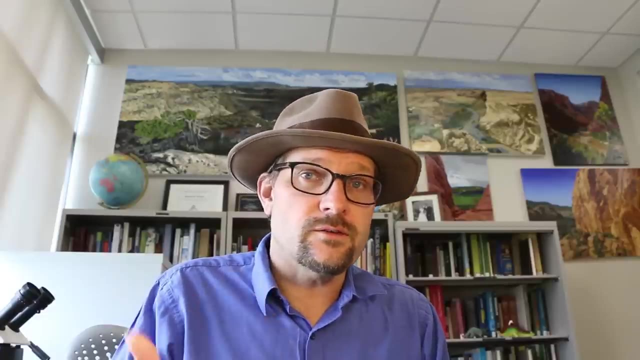 Now, specialized classes in paleontology related fields might be offered And you might consider taking them if they are offered. These include things like phylogenic systematics- that's kind of the organizing of organisms, how you organize organisms and classify them- Biostatistics. 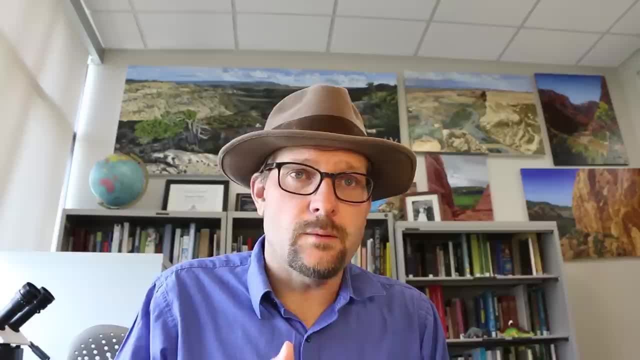 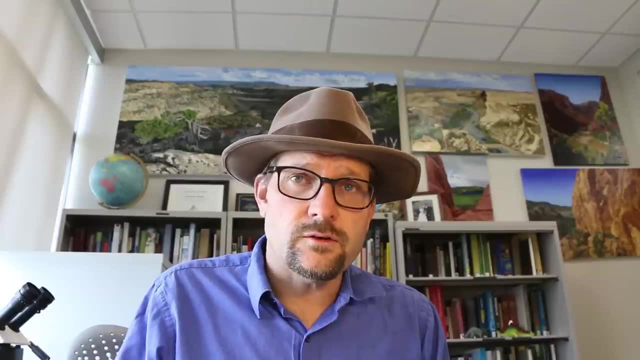 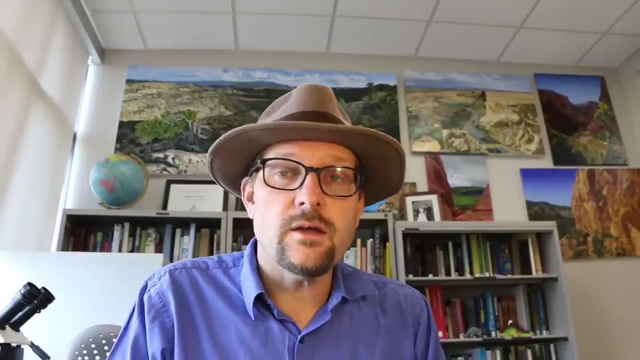 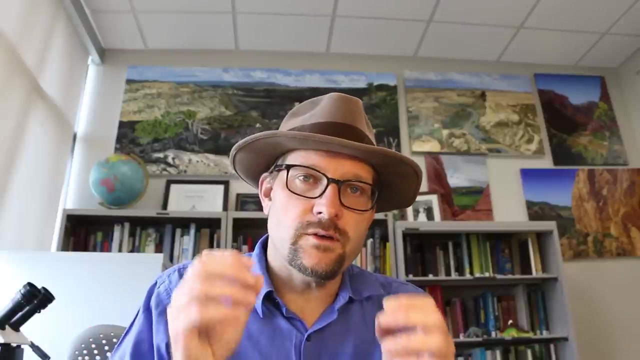 Geographic information systems or map making, cartography, scientific illustration, museum curation, functional morphology, biomechanics and other more advanced topics that are kind of specifically related to what you are interested in. You might also see if there are very specific paleontology courses offered, like mammalian. 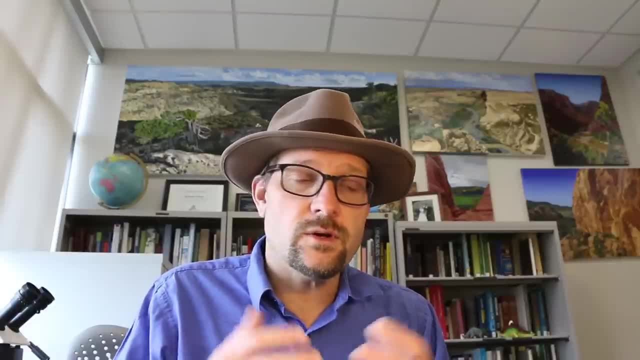 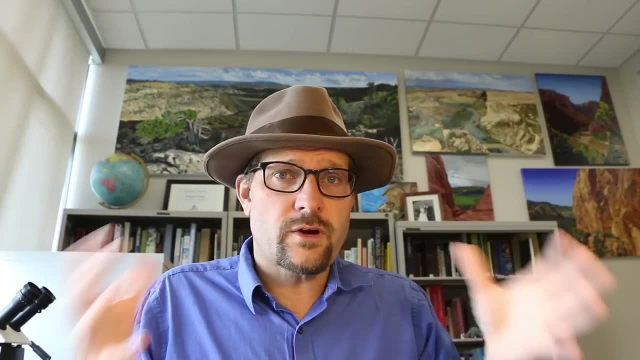 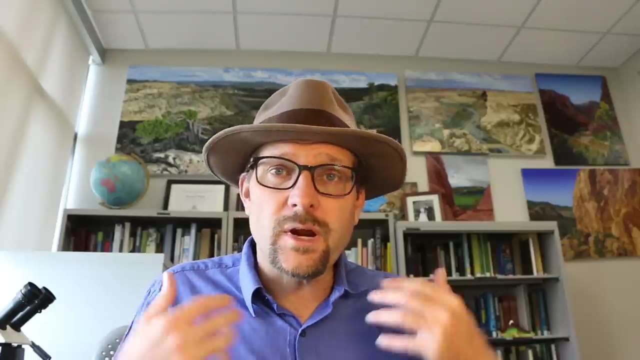 paleontology, or courses on dinosaurs, And if you are interested in fossil plants, of course, take botany and paleobotany. So, basically, what you are doing is you are filling your transcript with as many courses related to paleontology that you can find and you find interesting. 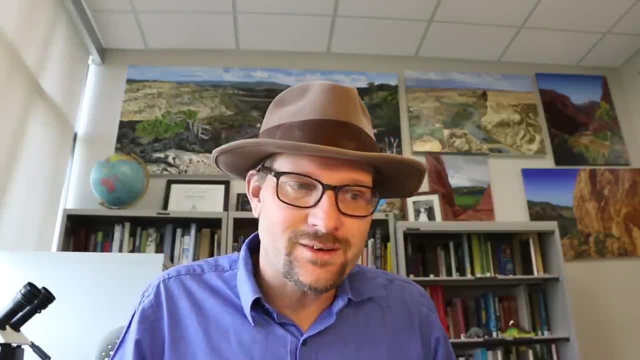 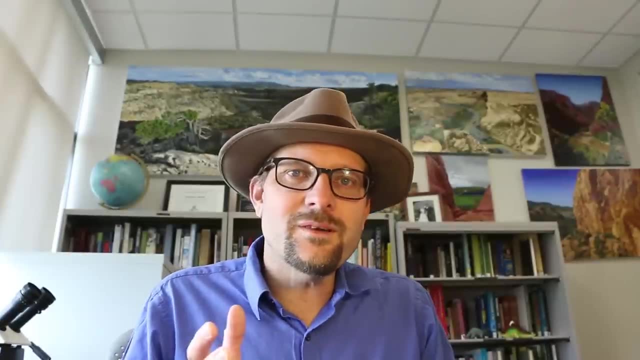 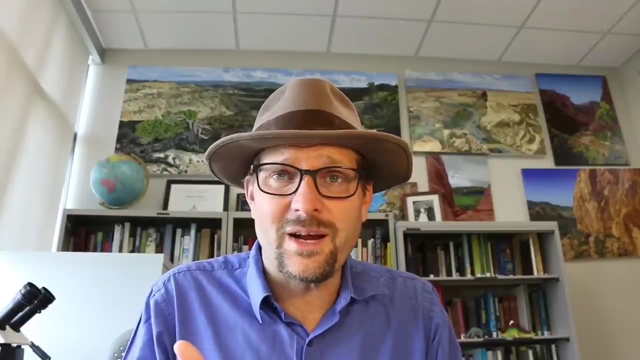 In my own education. I took most of these courses. I also volunteered at the University Museum and I spent my summers digging at fossils with graduate students. I remember one of my professors asked me: where are you going for graduate school? And I was like, oh gosh, what is graduate school? 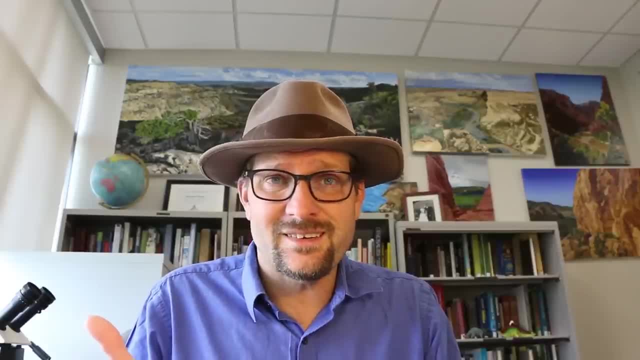 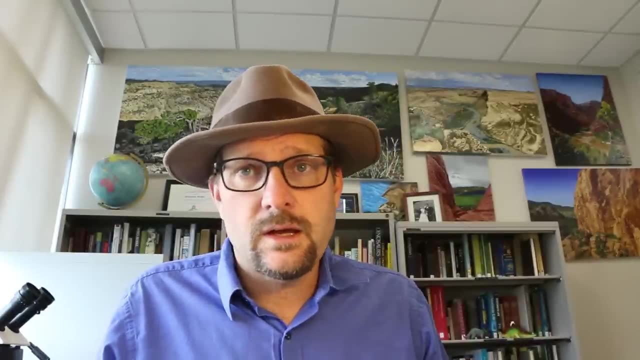 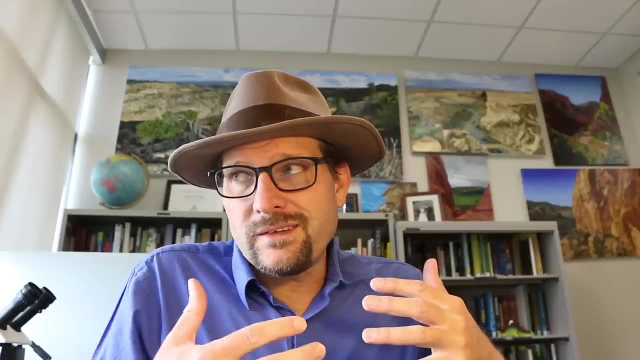 You know I had spent four years studying and it was like not over yet. So most jobs in paleontology require a master's degree in the field. To get a research permit here in the United States you need a master's degree, So it's kind of important. it's a very important thing to think about as you pursue your education. 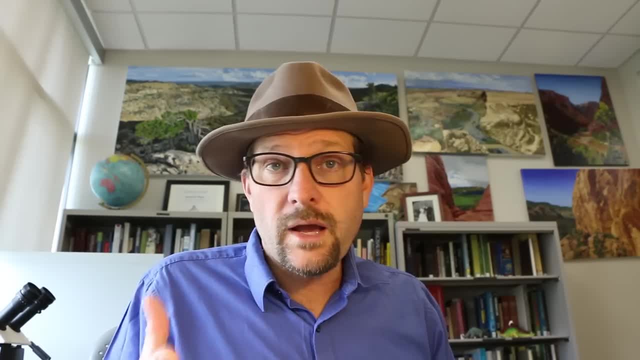 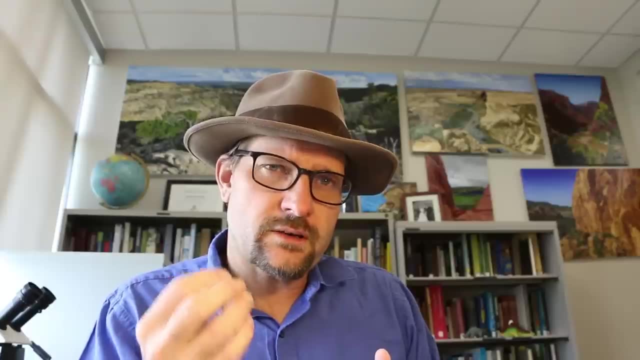 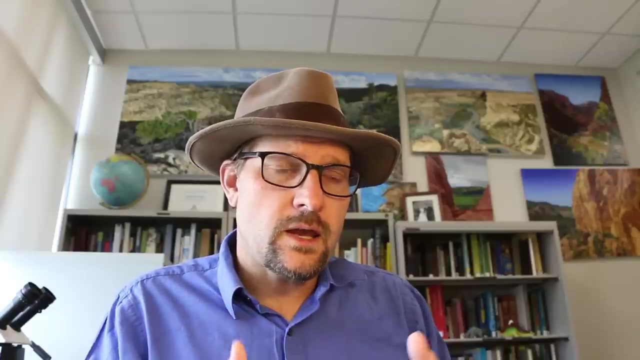 is where to go for your master's degree Now. a master's degree is a two to three year program, often with a very specific research project and advisor that you work with. You still take classes, but you also work on a research project that you lead and you 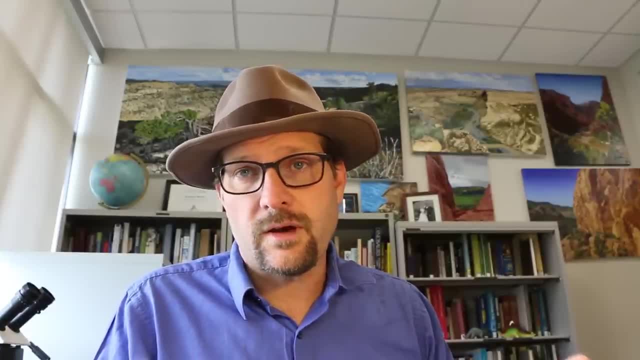 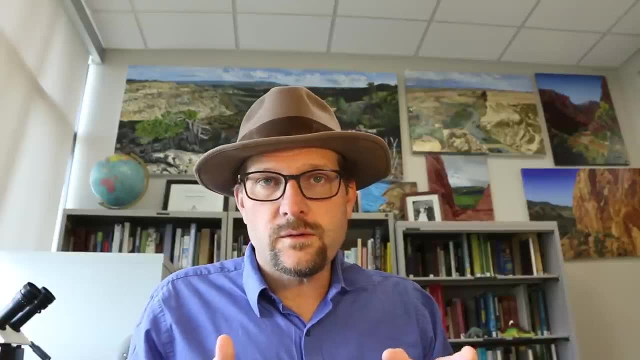 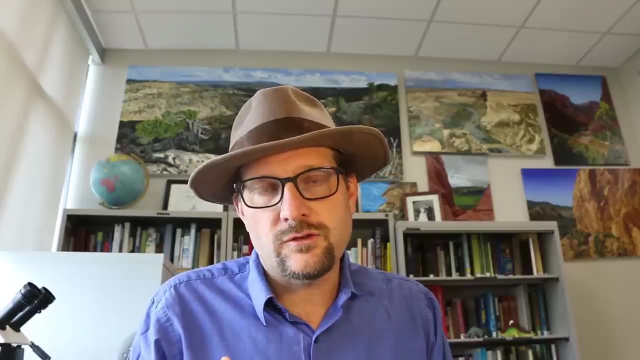 defend your research project in front of a committee of three to five professors. Now, not all universities are the same and some differ in their requirements. Here at the Uinta Basin campus of Utah State University, where I teach, we offer a master's degree in geology called the Applied Environmental Geoscience or AEG program that I mentor graduate. 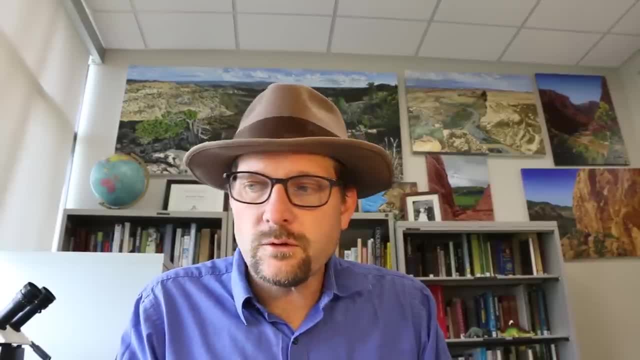 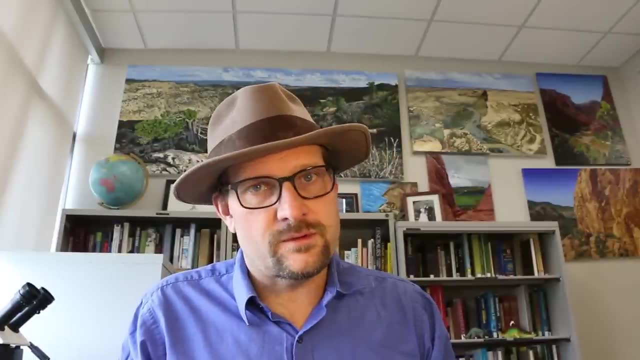 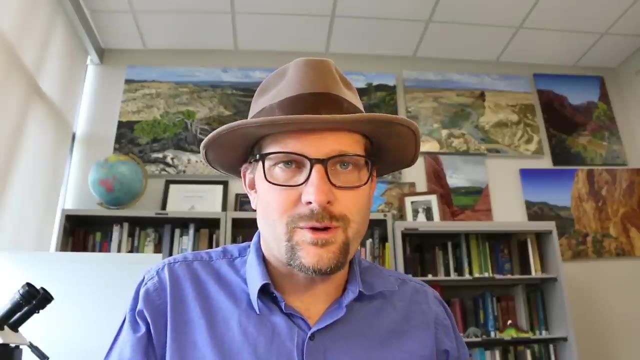 students who are interested in paleontology but also related geology fields, and it's a two year program. It's a fairly course, intense program of study. Applying to a master's degree program is more like applying to a job than to an undergraduate program, because often you're applying to work with a particular advisor or professor and 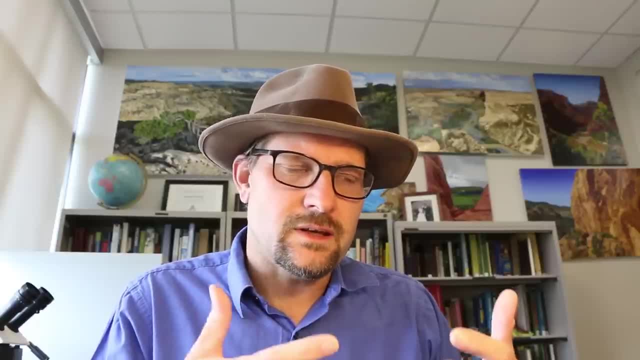 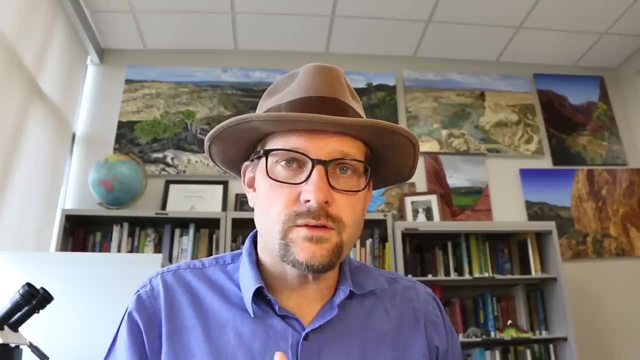 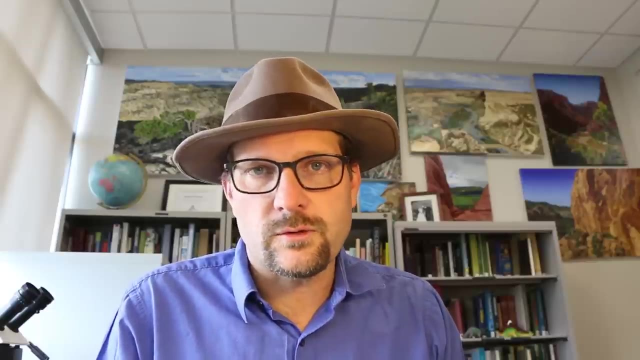 the best fit, not only in specialty and interests, but also personality and support for you as a student. Fewer students are accepted, so it's much more difficult to get into a master's program than it was getting into an undergraduate program. Apply to fellowships. 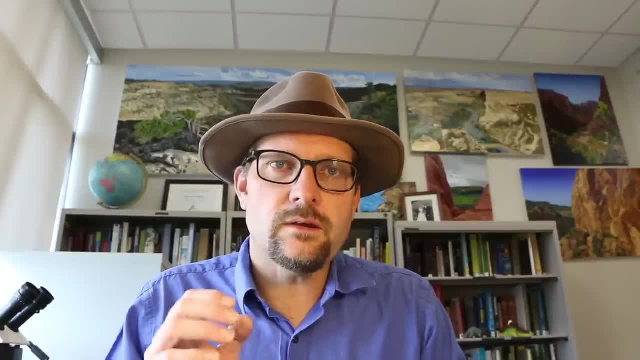 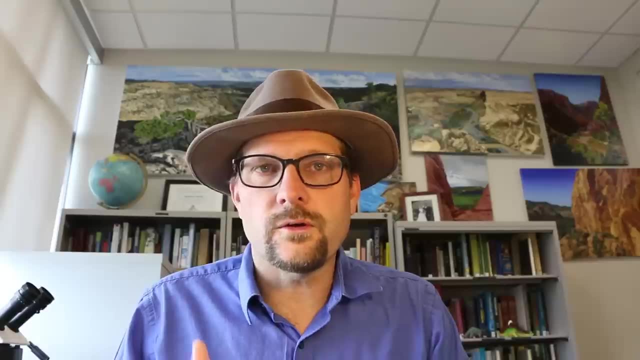 Often, what limits acceptance numbers into graduate schools is the available funding at each university. Since graduate programs are limited, You can apply to a master's degree program, but it's much more difficult to get into an undergraduate program. You're supported by grants or university teaching appointments. 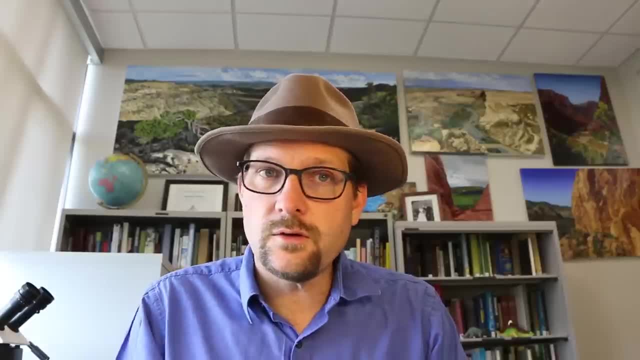 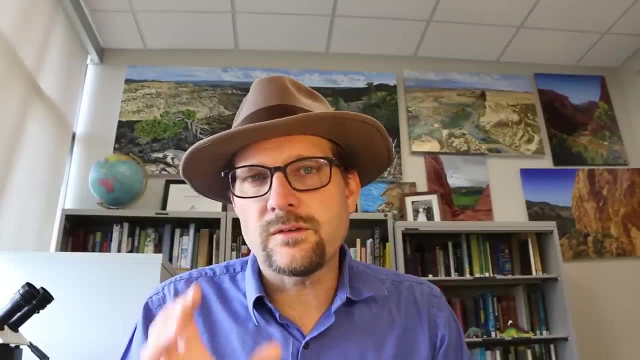 So if you have your own funding for research, a university would be more excited to accept you, since your project would be funded by your fellowship. But if you don't have a fellowship, you can still apply, as sometimes fellowships become available as you work through the program and apply to research grants. 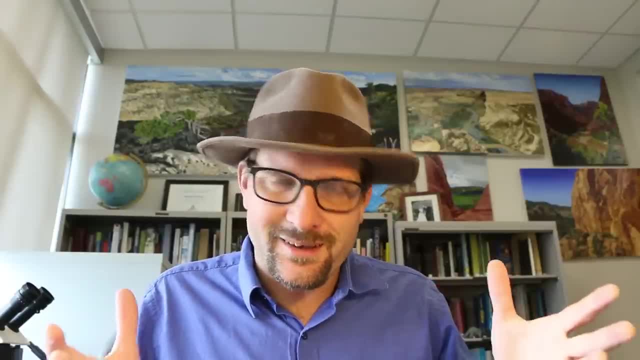 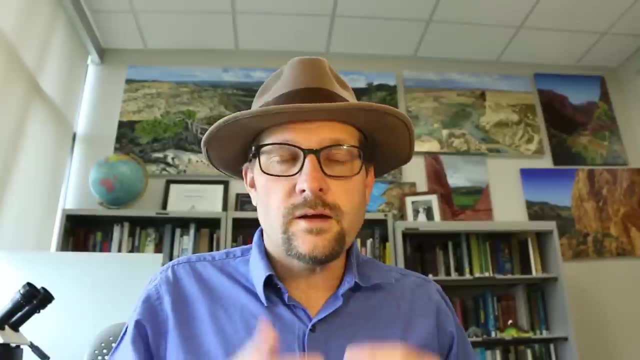 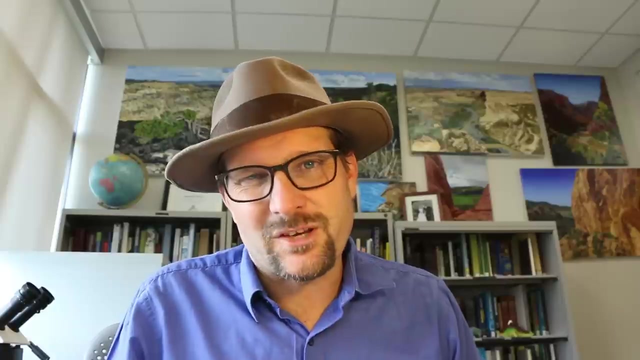 Now, after you have finished your master's degree, you have another choice, and that is whether to go on and do a doctoral degree Or seek out a job at this point Now. doctoral or PhD degrees are useful if you are interested in an academic job in the 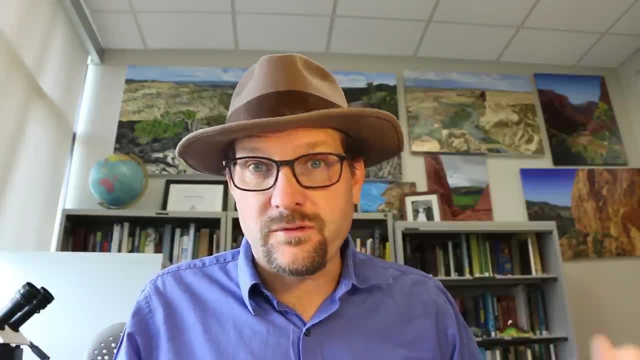 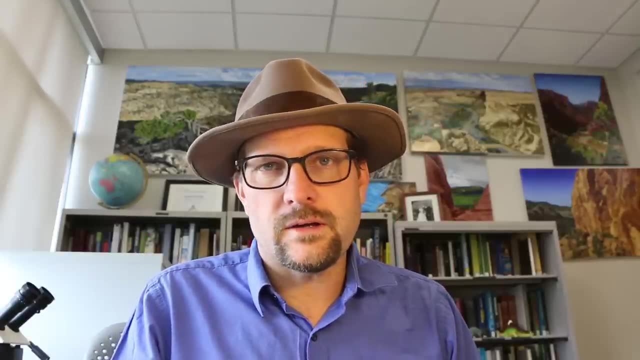 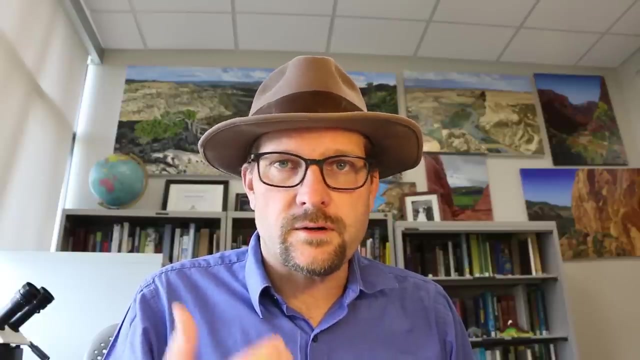 field of paleontology, particularly if you want to be a college professor. Doctoral or PhD degrees are also helpful in applying to grants and funding to support your own research projects, as you can serve as a PI or principal investigator on various government grant applications. 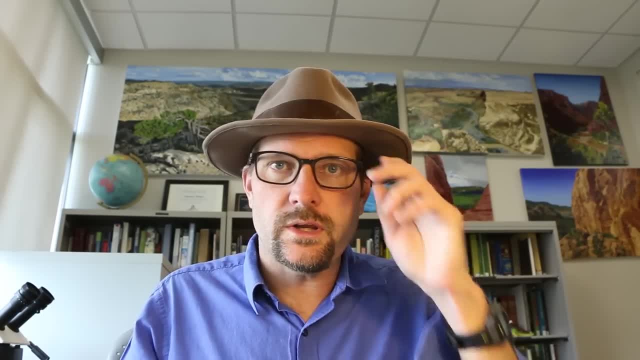 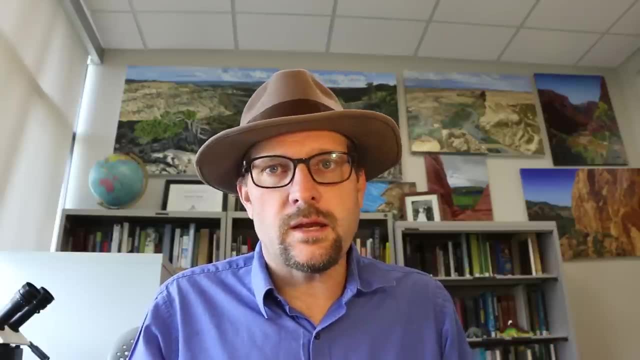 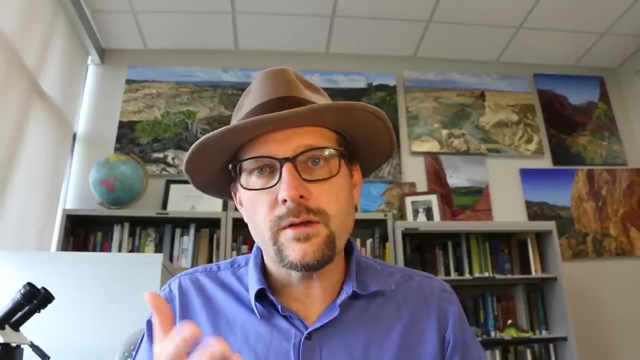 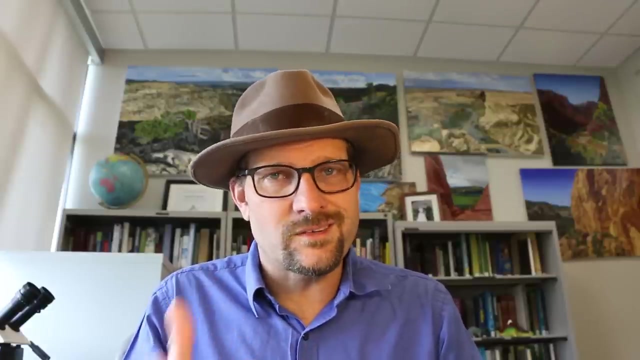 However, having a master's degree will get you into the door of most jobs in paleontology, but may limit your advancement later on, depending on your institution and or company. So some places, like universities, highly value PhD degrees, while other institutions like private companies, museums and non-profits tend to value experience and talent more than. 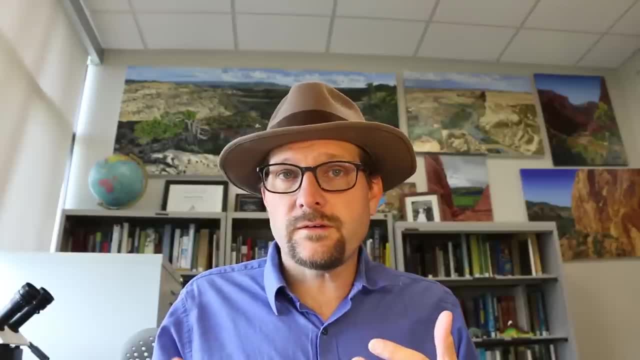 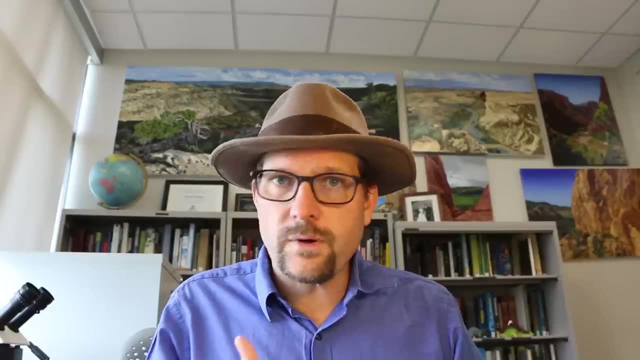 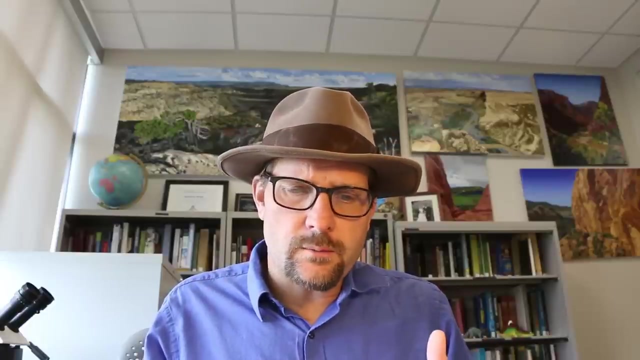 having a PhD added to your name. Now, I took five years after my master's degree before I returned for a doctoral degree. I probably could have worked the rest of my life without a doctoral degree as a paleontologist. However, I really wanted to do my own research and was spending all my vacation time out. 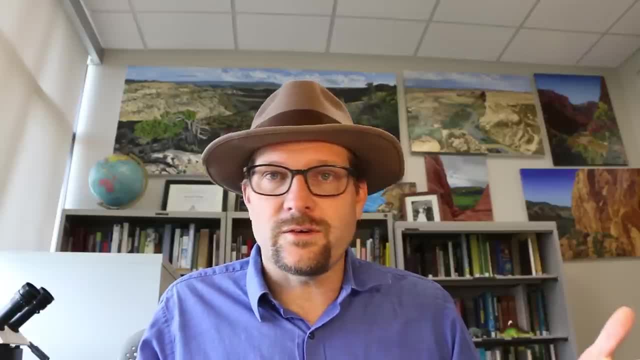 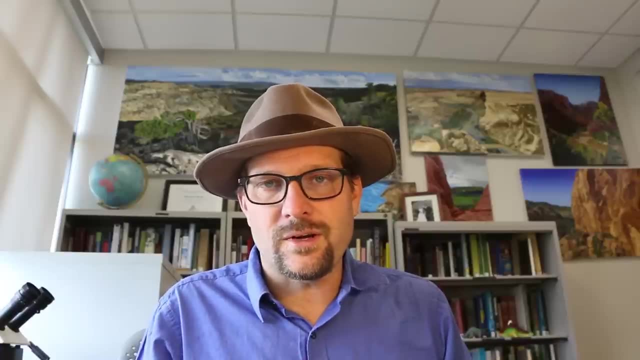 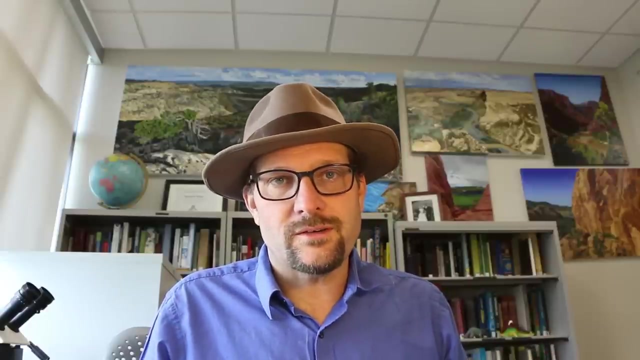 digging fossils, and I wanted to lead my own research expeditions rather than tagging along with other projects dependent on other people's funding. Having a doctoral degree was a requirement of my current academic teaching job here at Utah State, So consider this a possibility, especially if you want to continue on in academia. 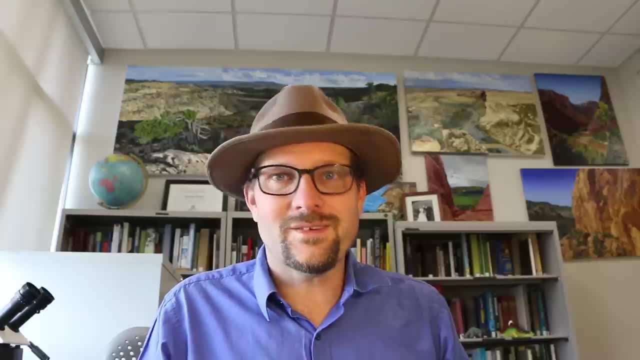 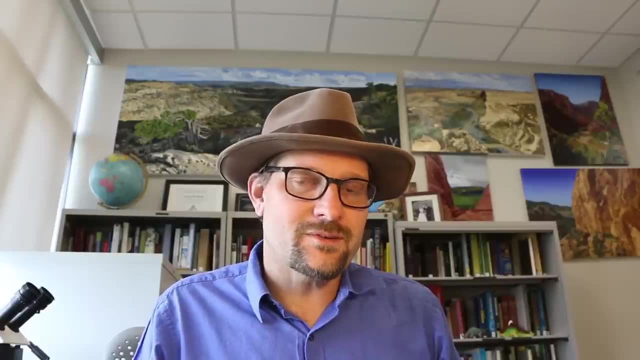 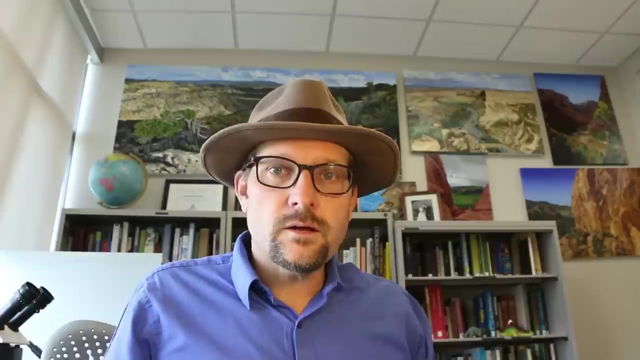 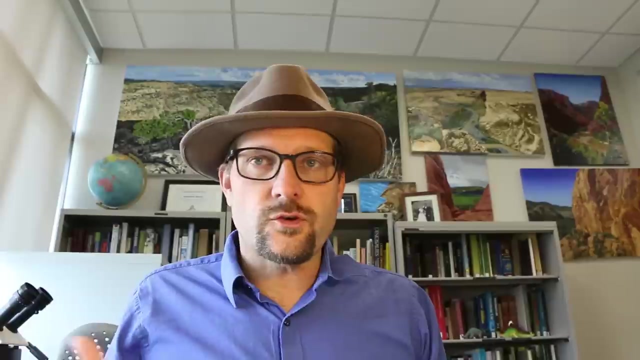 However, getting into a doctoral program is twice as hard as a master's program, and it's a big decision, since the average program of study lasts from five to six years. This is why professors are mostly Old people. Now, research done while pursuing a doctoral degree often defines your later research career. 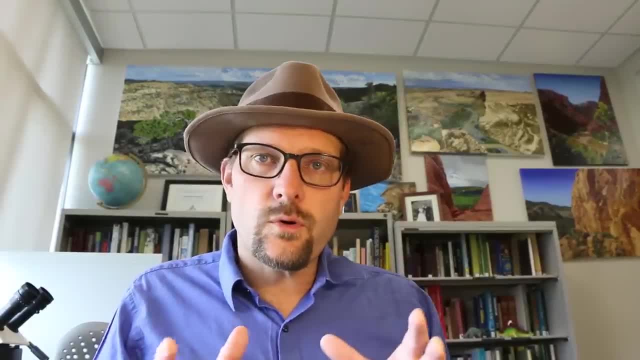 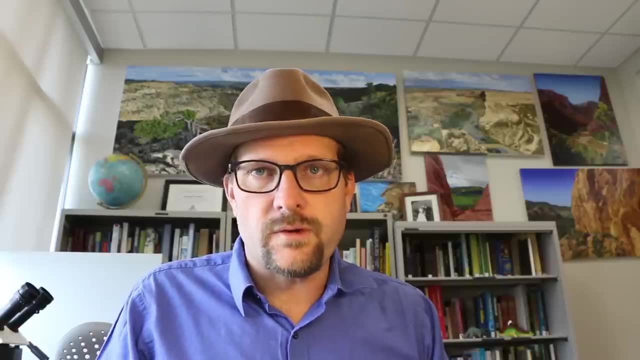 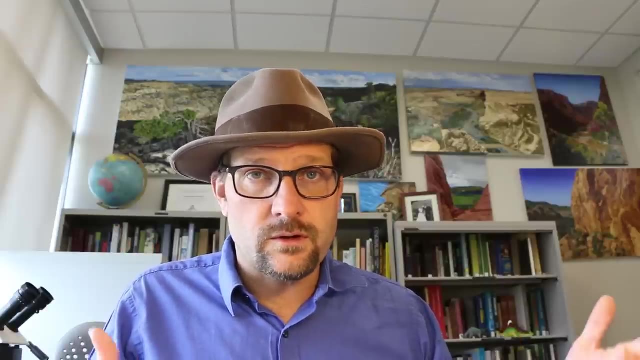 but not always. However, during that program you write basically a massive book, a dissertation, which you defend in front of a committee of five professors. If you're doing fieldwork overseas or leading an expedition into the field to collect fossils, you expect this research to take years to complete. 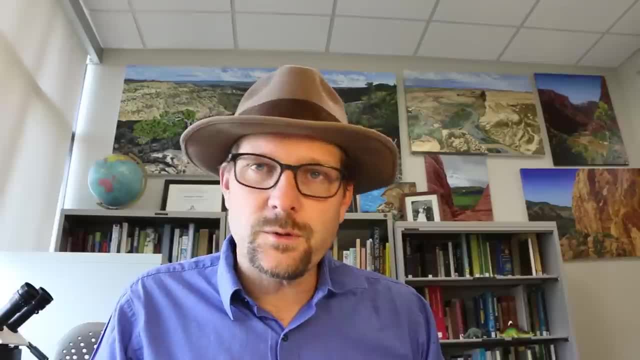 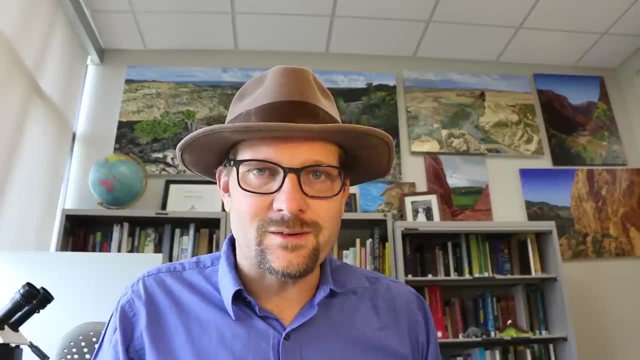 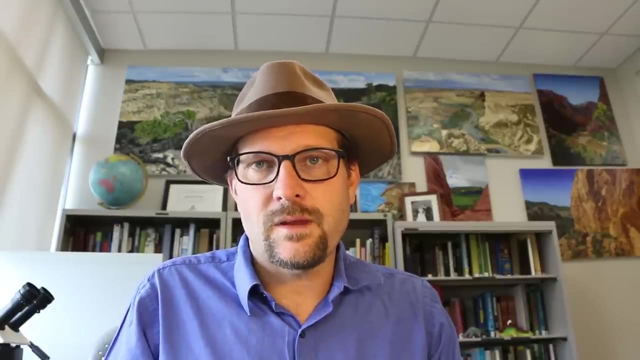 However, the experience is a lot of fun, really rewarding, and especially if you're really interested in leading your own research project and you're very disciplined. After a PhD degree, a post-doctoral job may be an option. This is where a funded research project- often it's a large museum or university- is looking. for additional experience, People to join their research projects, And for them, a PhD is the most important option, So they can do their research. I'm going to give you an example, But let me give you a few examples. I'm going to give you a few examples. 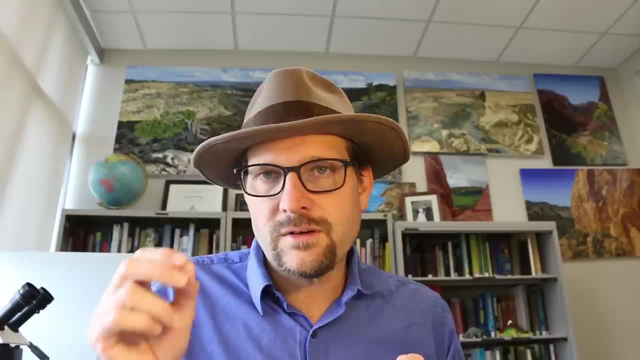 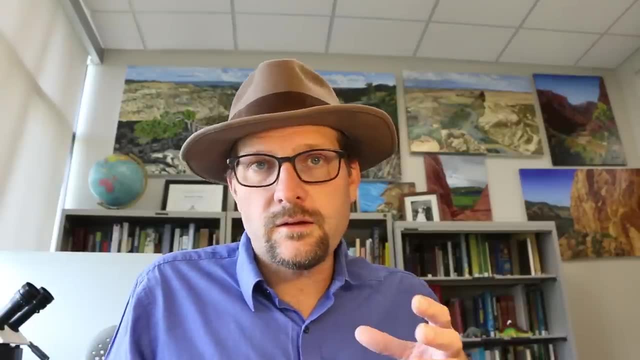 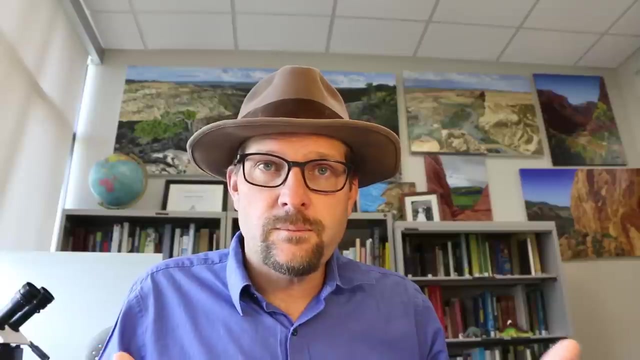 team on a particular project. These are time-limited research projects that last about two years, but they may be extended if funding is available. In paleontology, this might be an opportunity to join an international expedition to some exotic location or a university or museum that is looking for highly skilled paleontologists. 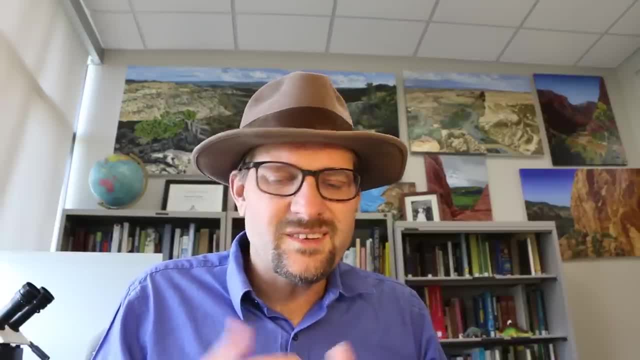 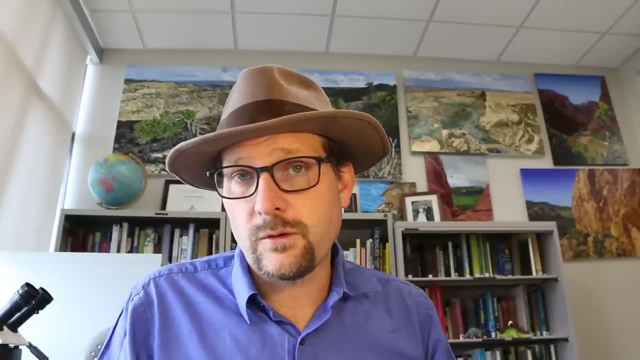 to join the crew for a project- They tend to be kind of rare in paleontology- most commonly offered by the big museums here in the United States such as the Smithsonian Institute, the Chicago Field Museum or the American Museum in New York City.